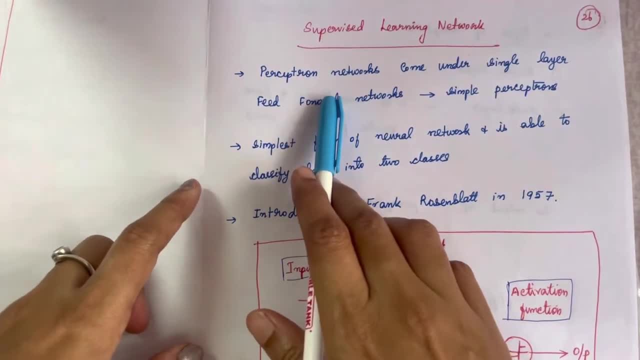 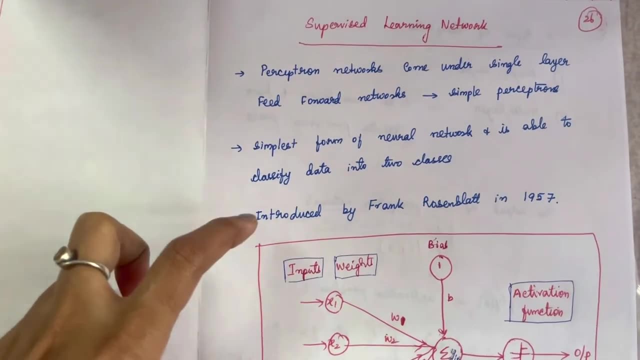 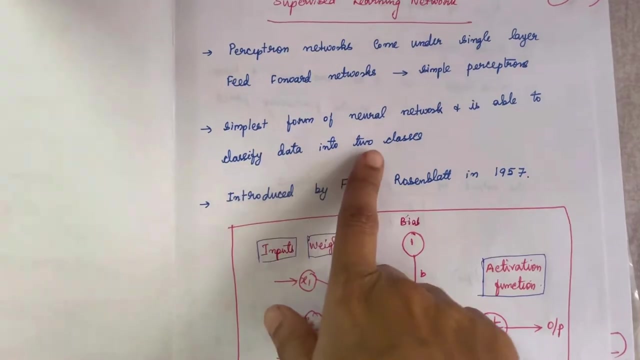 neural network too. Okay, so let's get into this video. So in this video, I will be explaining to you the architecture of perceptron neural network, the training algorithm and the flowchart. Okay, this perceptron neural network is mainly used for classifying the data into two classes. 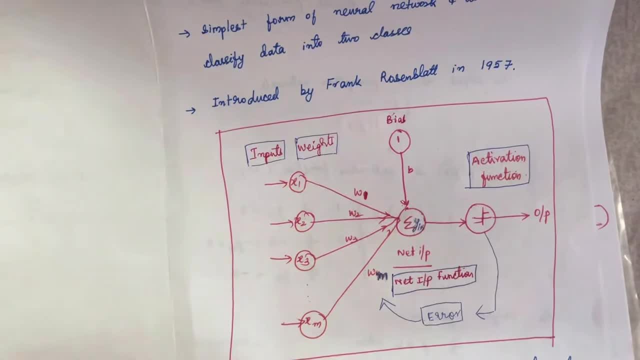 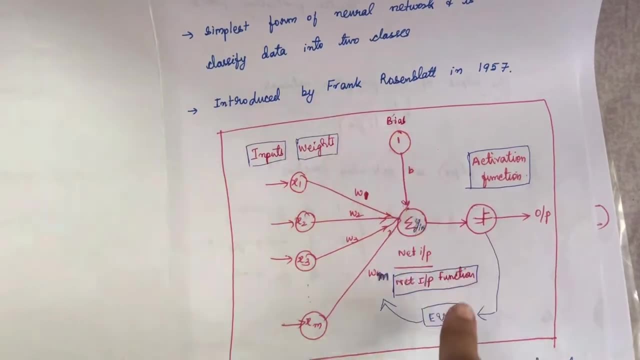 Okay, so the coming to this architecture of this perceptron neural network. there are four main parameters: One is inputs, the second is weights and bias. third one is net input function and fourth is activation function. So these are all the four main parameters. 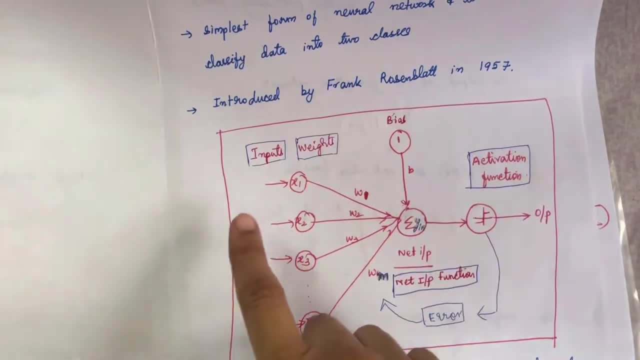 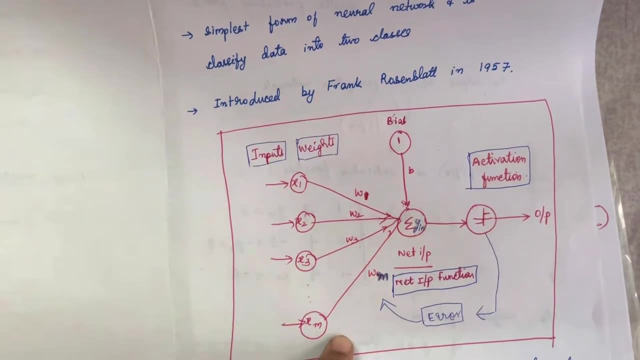 Which is which comprises of your perceptron neural network. First, coming to the inputs, inputs are nothing but the values, input values which are given to this perceptron neural network. Okay, so suppose, in your application if you are having four inputs, then there will be only four. 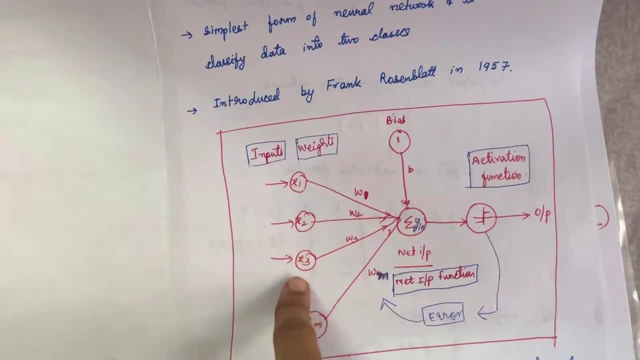 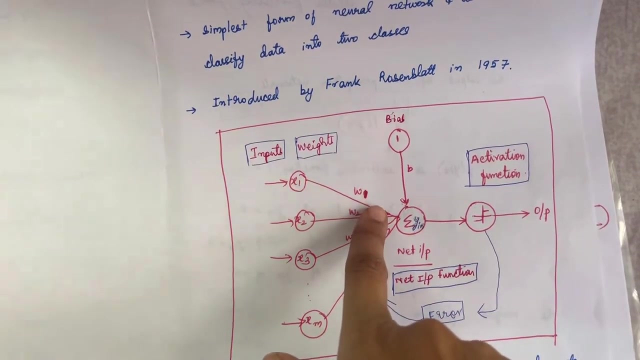 nodes: Okay, so, based on the inputs, you have to give the nodes. Next is weights and bias. So weights and bias are the values between the inputs and your output function. So these are all values It will have. it will take the value between 0 and 1.. Okay, so these are all the values. 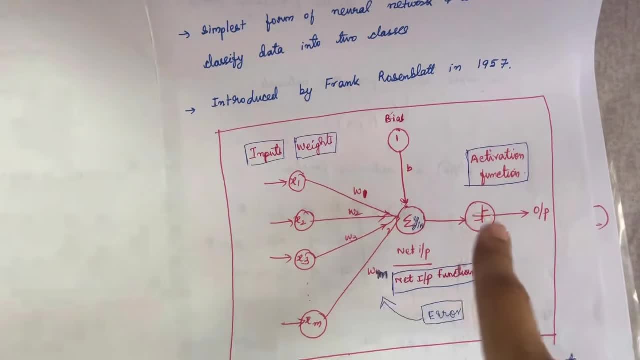 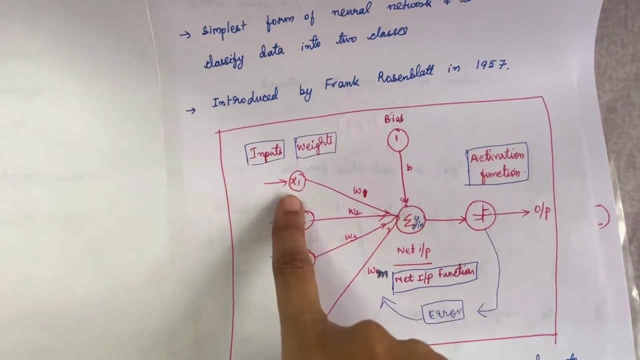 between your inputs and your output function. The next is net input function. Net input function is calculated by multiplying the input values and the weight values. Okay, so the formula will be x1 into w1, plus x2 into w2, plus x3 into w3, etc. up to xm into wm plus w2 into w3.. So this is the 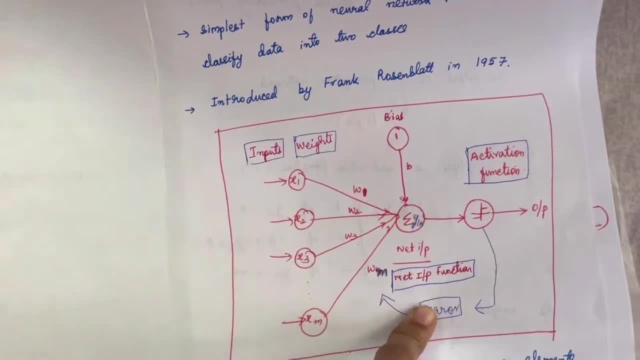 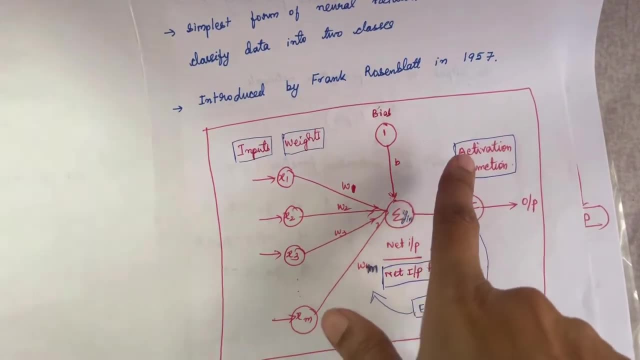 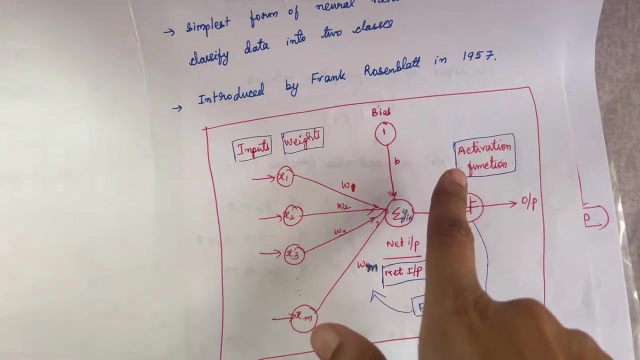 1 into b. that will give you your net input function. After calculating net input function, you have to apply your activation function. Activation function will help you to tell whether the neuron is going to fire or not. So there are many activation functions available. 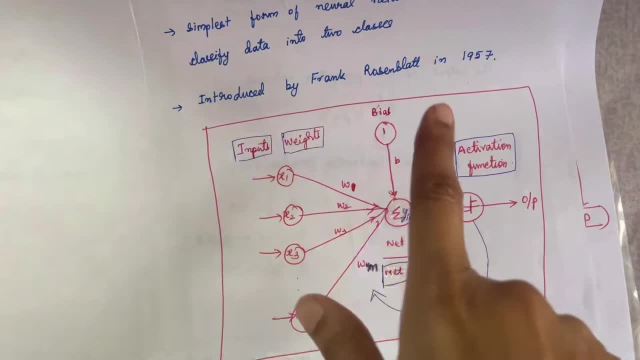 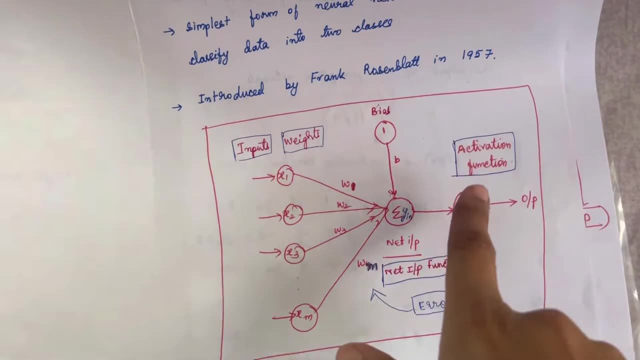 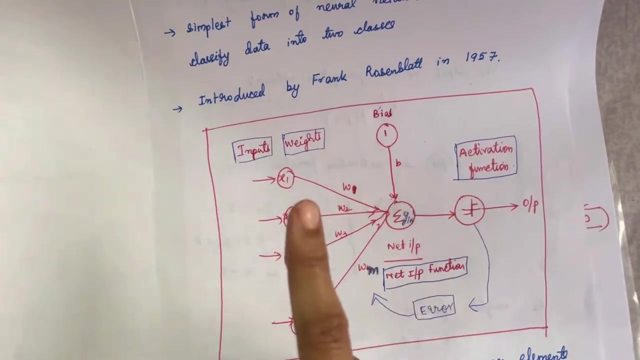 So in this perceptron neural network, Mr Frank Roselbert, he used step activation function. So here after applying the activation function you have to apply the activation function. So in this activation function you will get the output. This output value is compared with the target value. 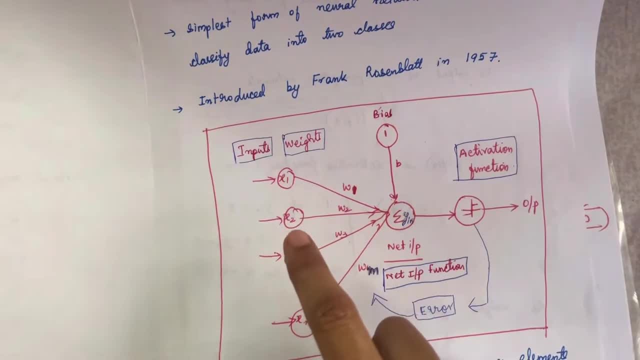 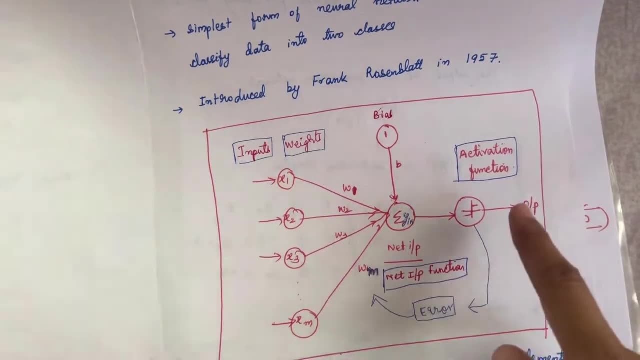 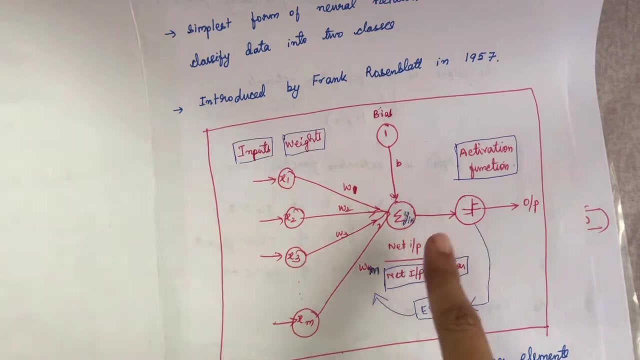 So we, as I have already told you, this perceptron neural network is a supervised learning model where both the inputs and the target values will be given. So the output values which you have received from this particular network is compared with the target values. Okay, 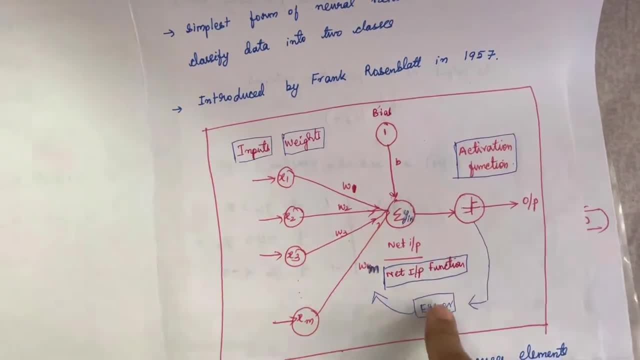 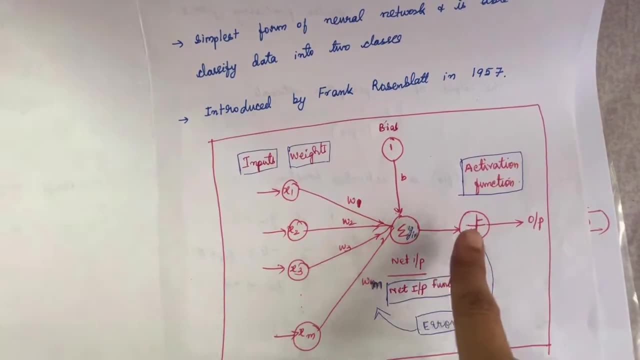 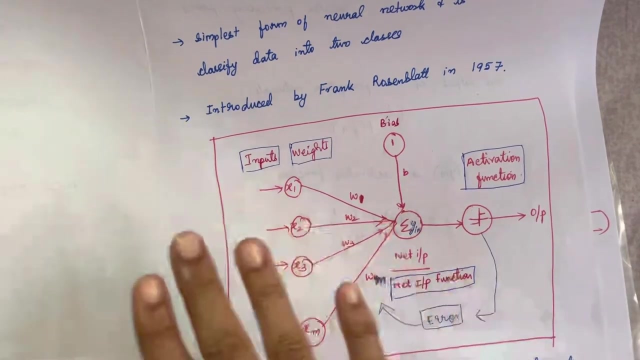 when you compare. if there is any error occurs, then again you have to train this network, You have to change their weight values and again you have to do the same process. So the same process will be iterated until there is no error in your network. Okay, this is what. 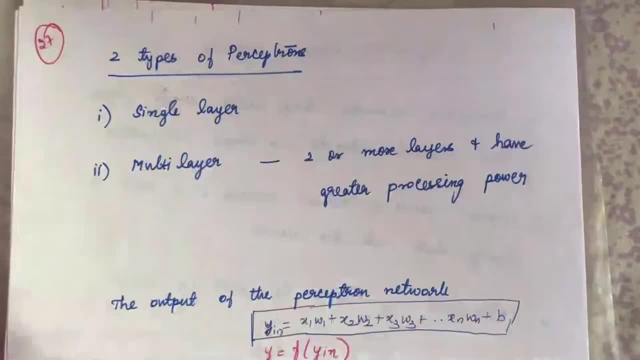 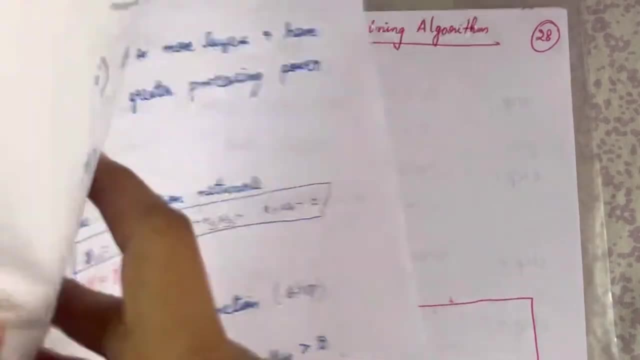 your architecture of your perceptron neural network. Two types of perceptron. One is single layer perceptron and multi-layer perceptron. Single layer perceptron is the perceptron architecture we have seen. There is only one layer, Okay, and you can also have multi-layer. 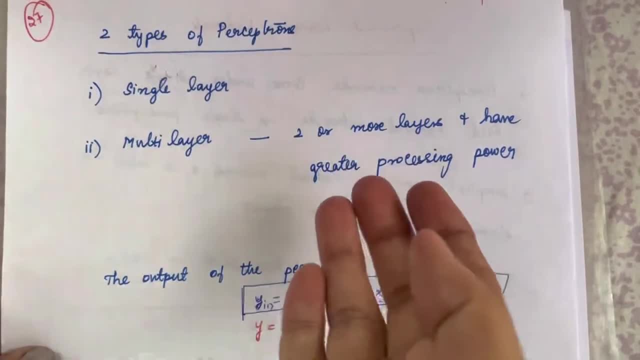 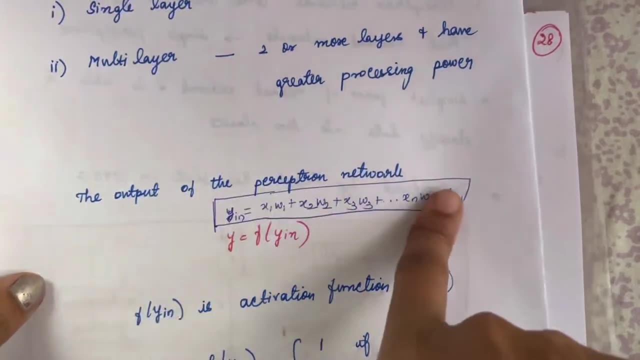 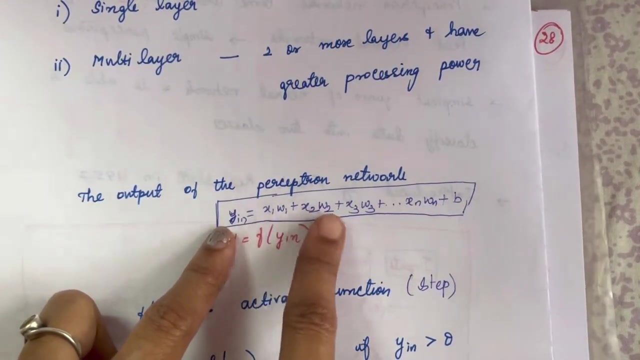 perceptron. This means that there will be two or more layers will be there, and this will be used when you want to have a greater processing power. Okay, so the output of perceptron network will be like this, So we will call it as Y input. Y input will be equal to X1, W1 plus X2, W2 plus X3 W3. 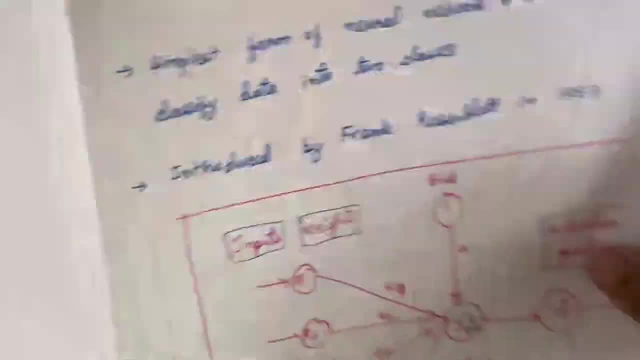 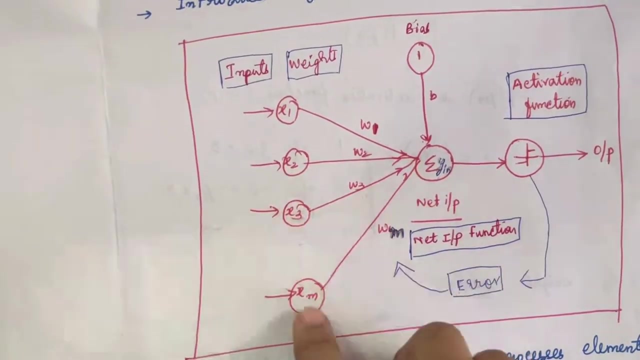 plus, etc. up to Xn Wn plus 1 into B. This is nothing but the Y input, Y input. how you are getting this Y input: X1, W1,, X2, W2,, X3, W3, etc. up to Xn Wn plus 1 into B. That will be your Y input. 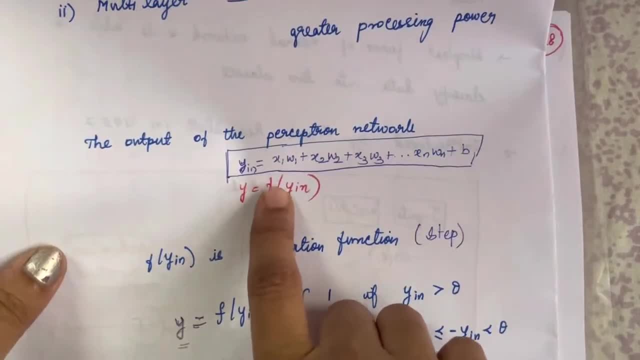 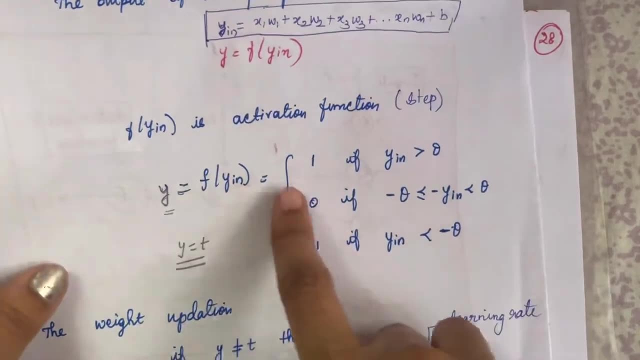 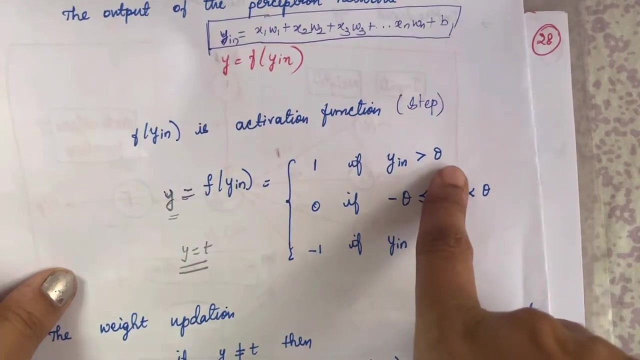 After calculating Y input, you are going to apply the activation function F of F Y input. you are going to get Y. So what is this F of Y input? This is the activation step activation function. So F of Y input value will be 1 if the Y input value is greater than some threshold. So 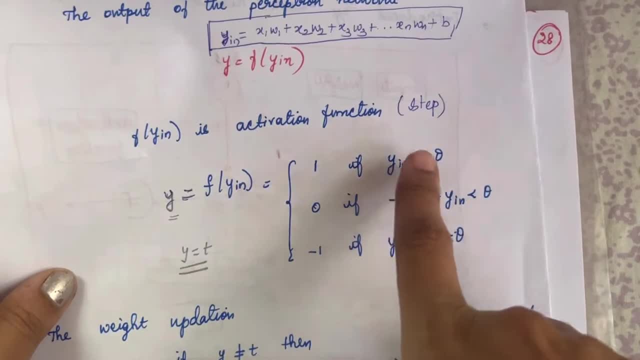 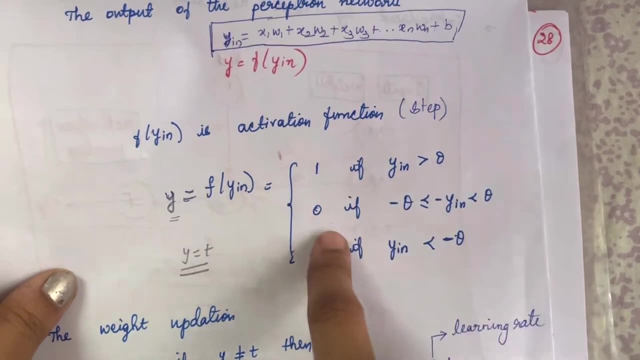 you have to keep one threshold. If that, if the Y input value is greater than the threshold, then the output value will be 1.. If the Y input value is between minus theta and plus theta, the value will be 0. And if it is less than minus threshold value, then it is minus 1.. Okay, 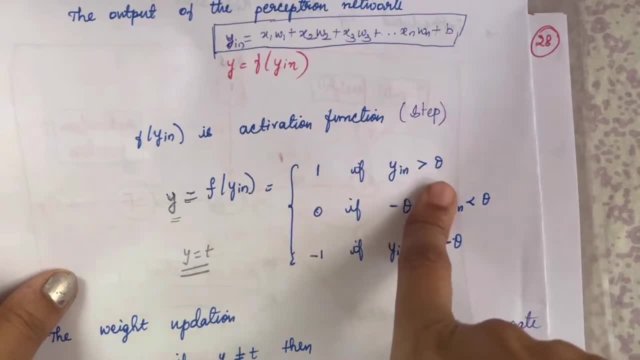 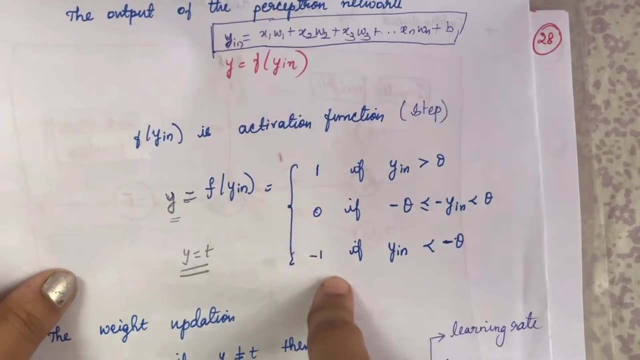 this is what the activation function you have to use. So when it is greater than threshold value, you have to set as 1.. If it is between minus theta to plus theta, you have to set 0.. If it is less than theta, you have to give it as minus 1.. So that is what your output value. So weight. 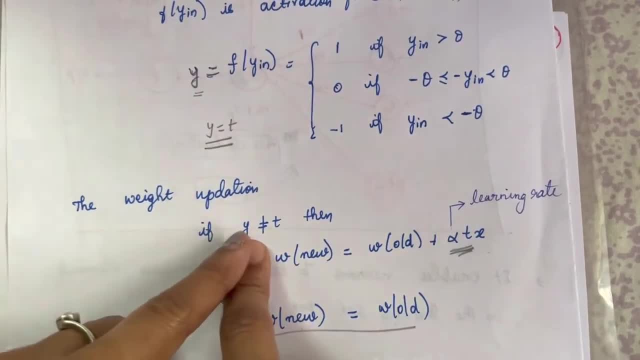 updation. how do you update the weights? It is based on the target value, So you have to compare the output value which you have received from the network with the target value. If it is not equal, then you have to update the weights So the new weights will be equal to. 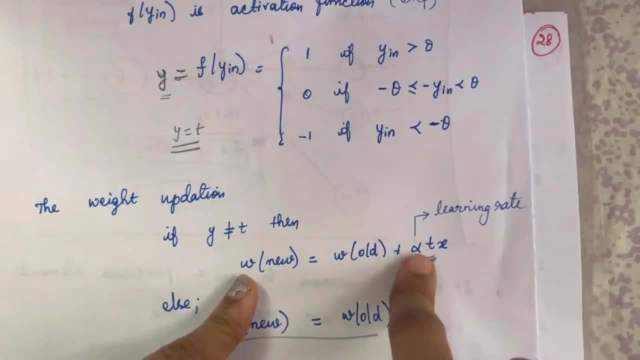 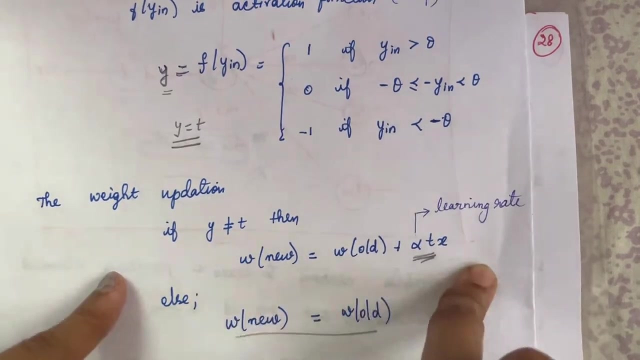 old weights plus alpha into T, into X. Alpha is the learning rate, So this will help you to learn that particular train, the network And it will be. the value will be between 0 to 1.. And T is a target value and X is the input value. So this is what you have to do, it for weight updation, Else. 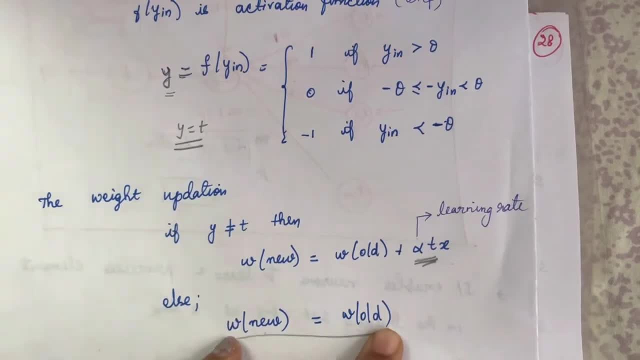 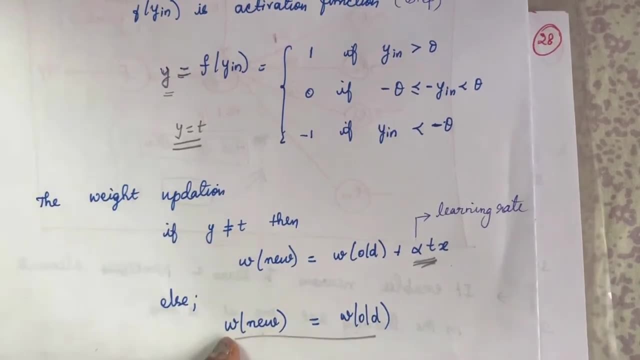 if they are not equal, then you have to update the weights, So you have to compare the output value between 0 to 1.. If both are equal means, then you have. you can set the old weights to be the new weights. That means that there is no change in weights, So you can take that as the final output. 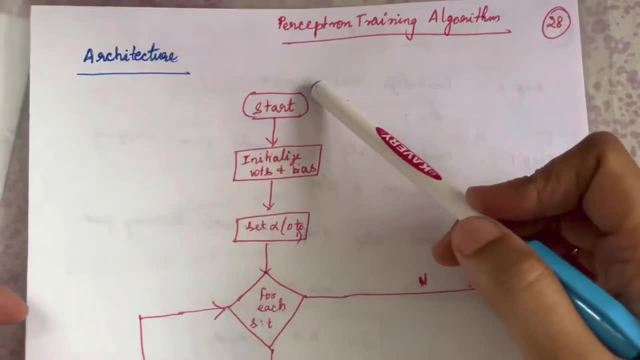 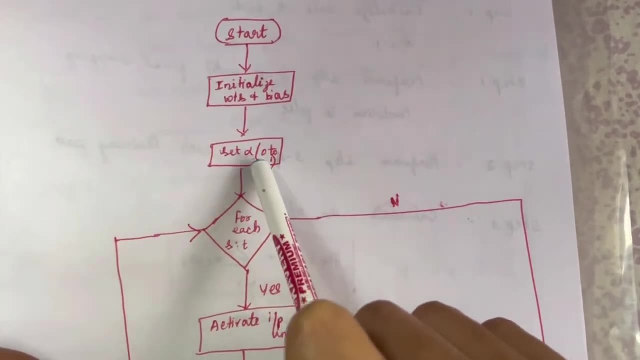 Okay, we will see the flowchart for this perceptron training algorithm. So first is start. Now we are going to initialize weights and bias and you are going to set the learning rate- that is nothing but alpha- to be 0 to 1.. And for each training input pair, so you are going to activate the 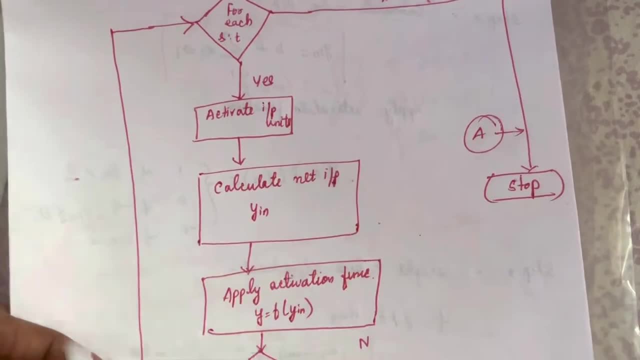 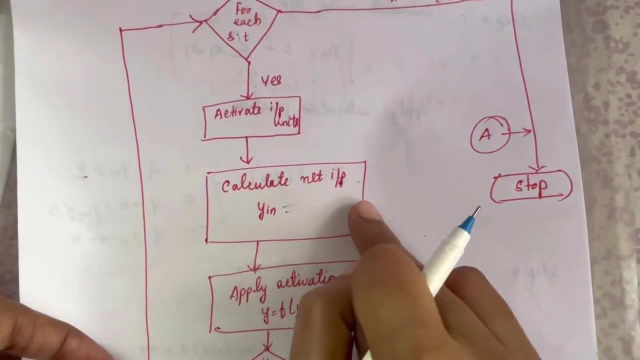 input units. then you are going to calculate the net input value. So you are going to activate the net input, that is y input. that is nothing but x1 into x1 into w1 plus x2 into w2 plus x3 into w3. 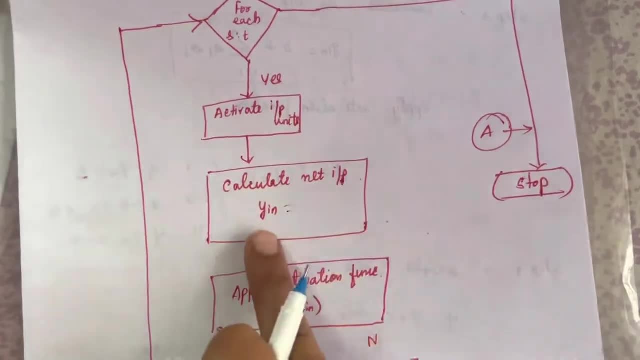 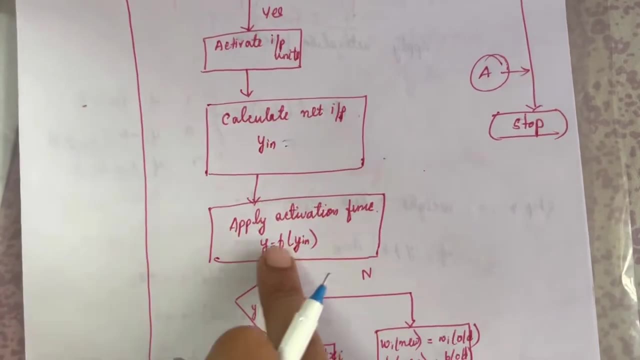 extra up to xn into wn, plus 1 into b. So then you are going to, after calculating this activation function, you are going to apply this net input, you are going to apply this activation function and you are going to get y and you are going to compare this y and t If this is equal. 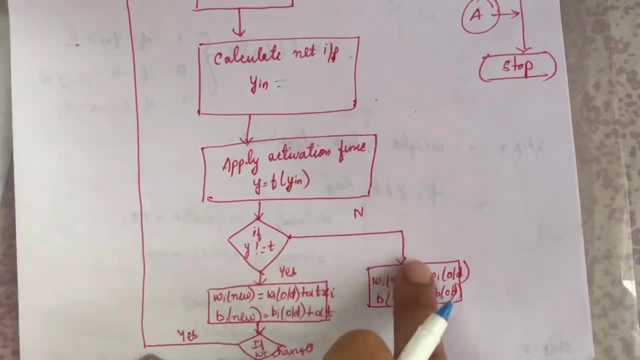 if this equal means- there is no change means- then you are going to set the old weights to be the new weights and old bias value will be the new bias value. If they are not equal, then you are going to apply this formula- old weights plus alpha, into t, into: 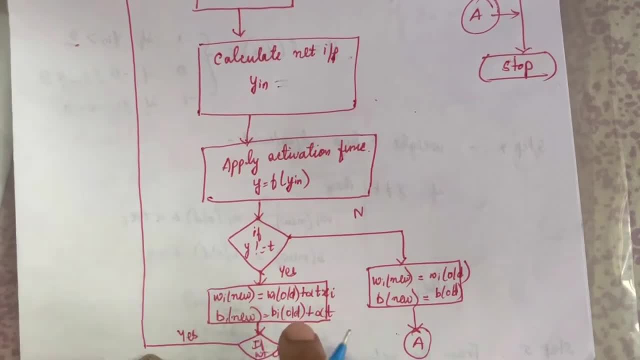 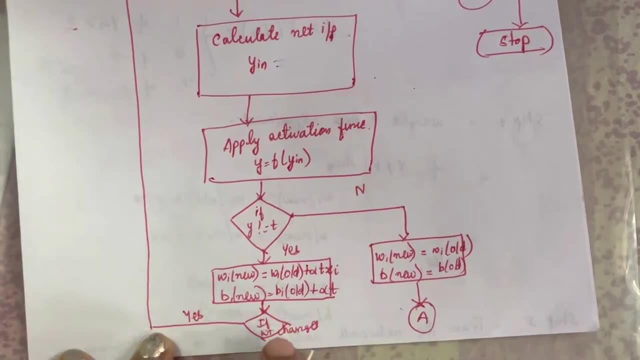 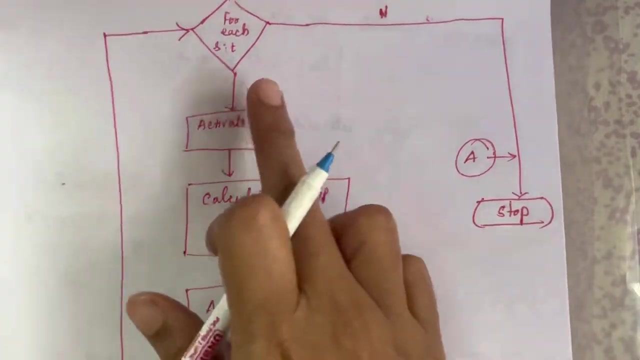 xi, that will help you to find out new weights and old bias value, plus alpha into t will help you to find out the new bias value. Okay, so then you are going to, if the weight changes means again you are going to proceed. this step, Okay, this is this step- is going to be proceeded. If not, 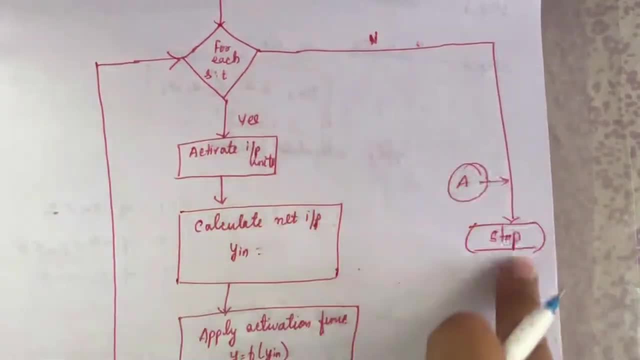 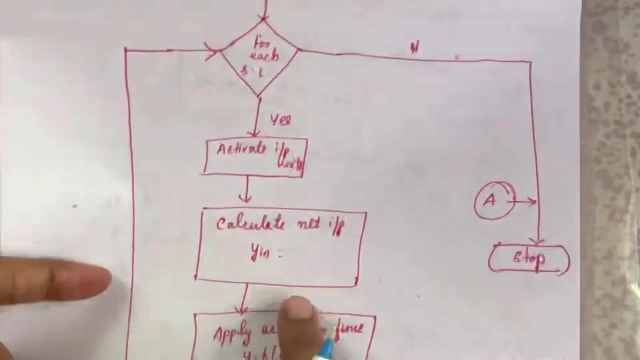 if there is no inputs- there is no further inputs- then you are going to stop this algorithm. Okay, this is a simple algorithm where you are going to: first you are going to find out this y input, then you are going to find out this activation function, then you are going to apply. 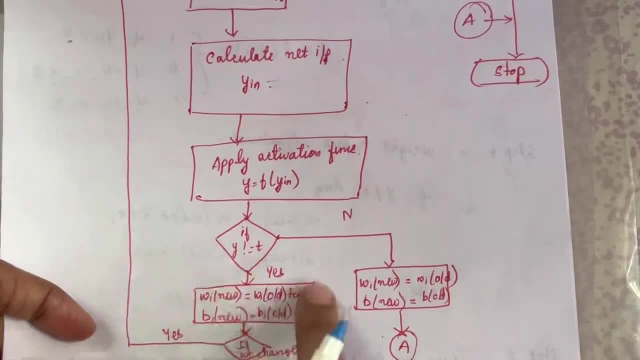 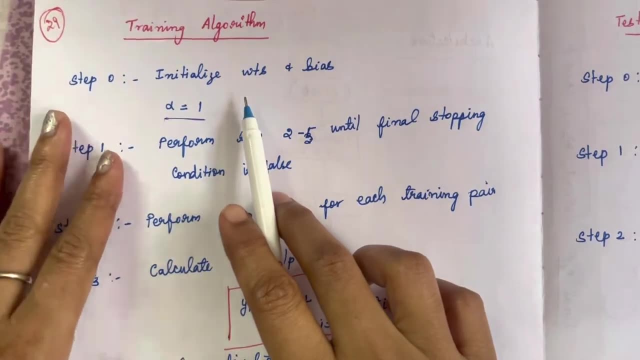 compare the y and t. If they are not equal, then you are going to use this particular formula. Okay, this is training algorithm. So, training algorithm. we will write this training algorithm based on the flow chart, the same what we have done in the flow chart. we are going. 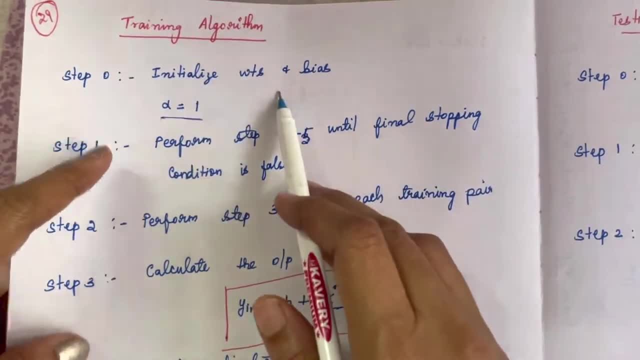 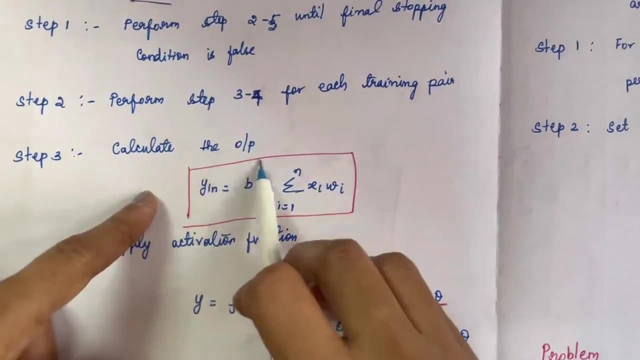 there is a 5uc situation where you will have a equation: Okay, you will update the function e for e to A for e to B. Now, let us say till after it isine 20, the input function points to b, from x to t, which is unknown, because in the normal way, what you are gonna need 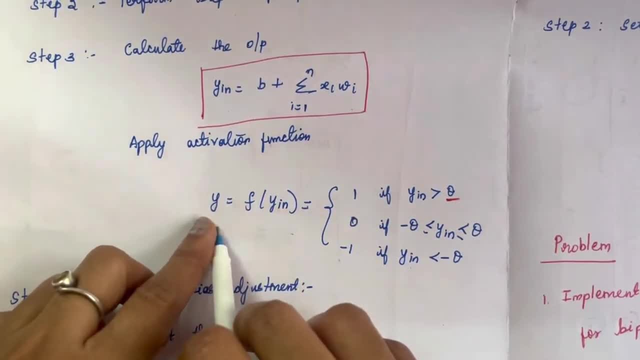 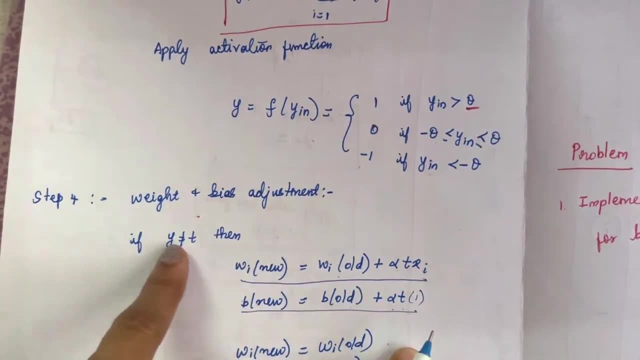 that is your pure infotable value. you are going to extend your value. okay, so that's how, that idea that I told you. so now this starts bringing back the how is there? So all you are gonna create this formula usingemoval y, because when it comes to step 10, we will. 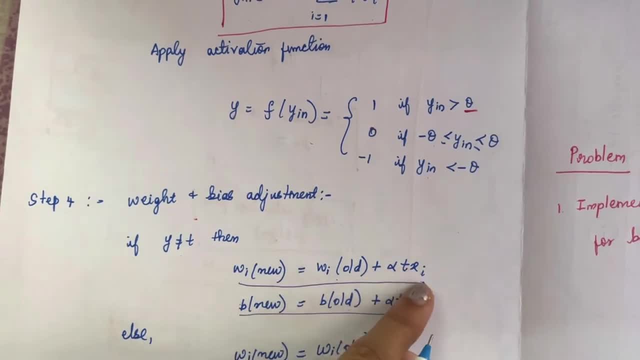 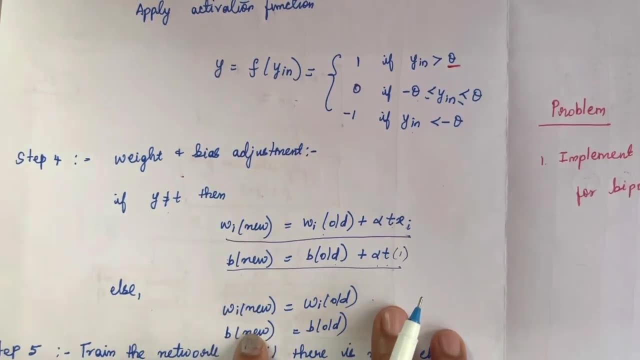 equal, then you are going to update the weights by using this alpha into 2, into xi, or otherwise you are going to have the same weights to the to be considered for your old weights, that is, new weights and new bias. okay, this is your training algorithm x coming to testing algorithm. so there, 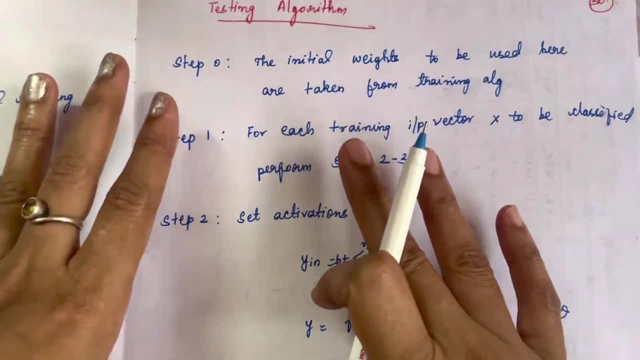 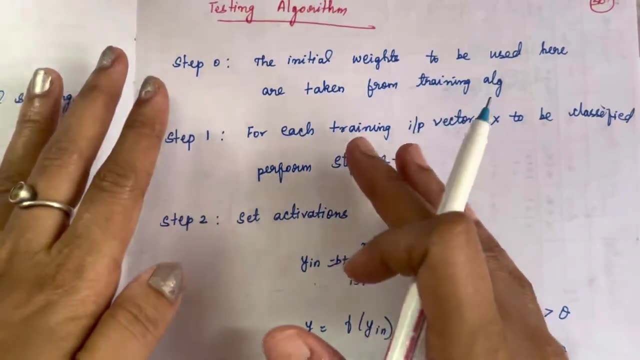 is always should be testing algorithm, because after calculating your weights, you have to check whether the weights you have received, you have got it from, the neural network is going to give you the proper output or not. that is why we need the testing algorithm. so for the testing algorithm. 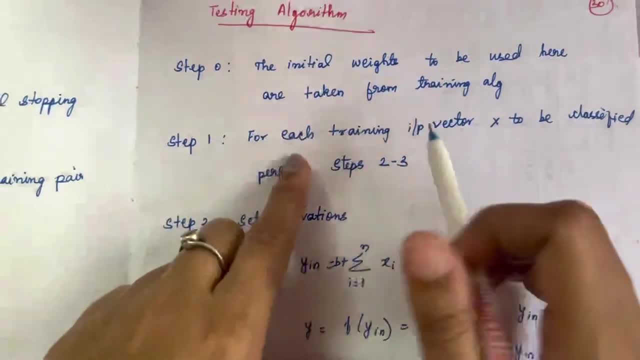 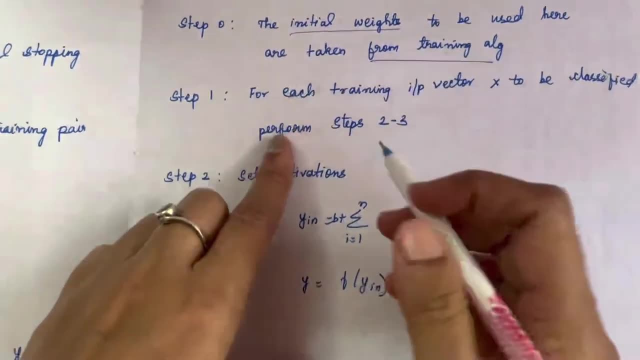 step 0 will be the weights. what you have received from the training algorithm will be considered as weights- okay, initial weights to be used here or taken from the training algorithm. and then you are going to, first, for each training pair, you are going to proceed this step 2. so step 2 is nothing.